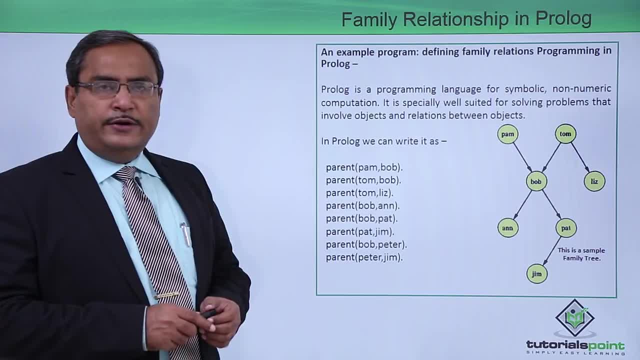 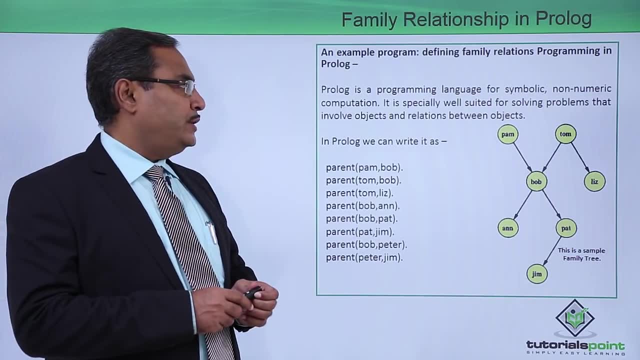 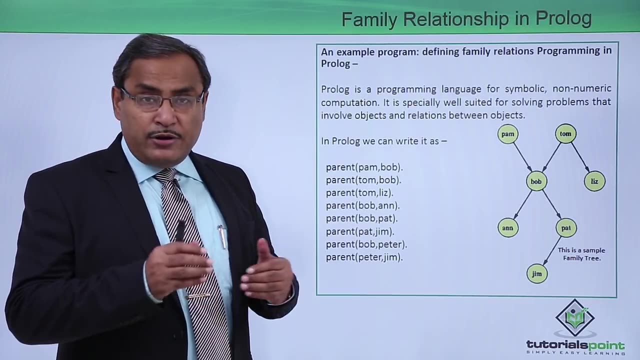 is Lij, So this is our family relationship tree. Prolog is a programming language for symbolic, non-numeric computation. It is specially well suited for solving problems that involve objects and relationships and between the objects and so on. So objects and relationships. 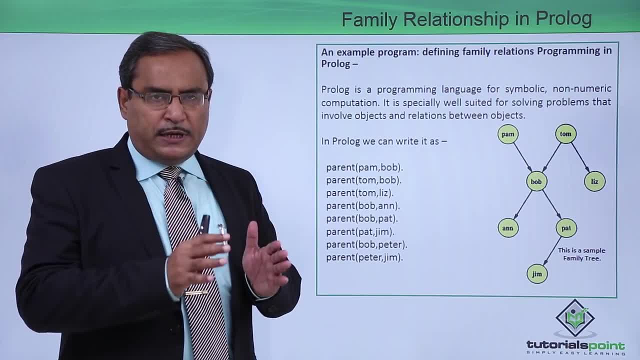 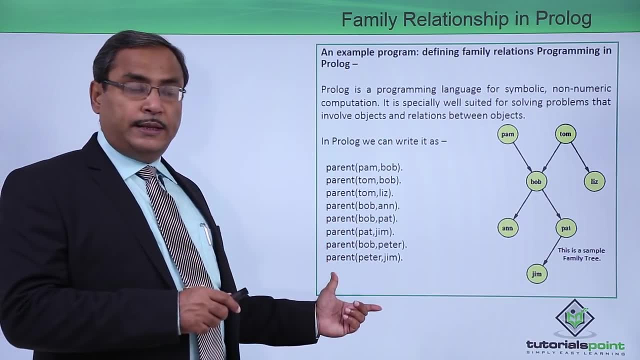 or relations between the objects will be depicted in our Prolog language. In Prolog we are going to show you that, how the family relationship can be expressed in Prolog. So in Prolog we can write this family tree as like this one. So parent Pam. 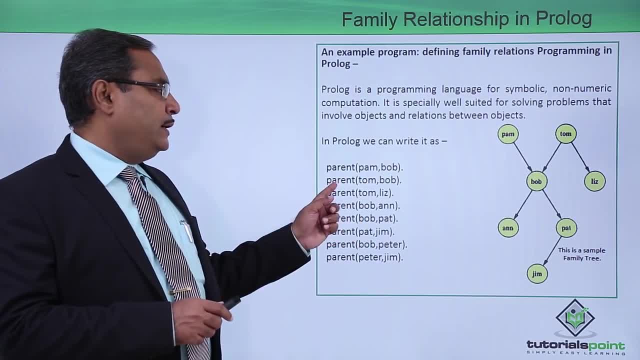 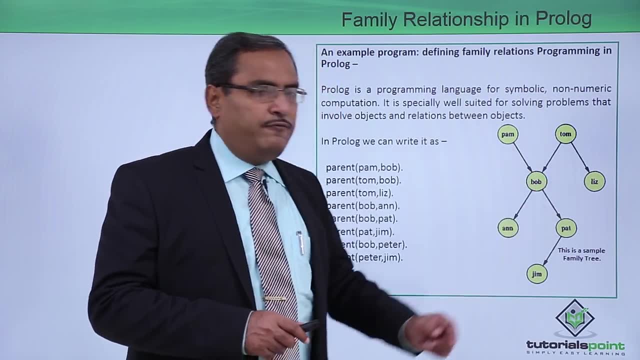 Bob, So Pam is the parent of Bob. Parent Tom Bob, So Tom is the parent of Bob. Parent Tom Lij, So Tom is the parent of Lij, and so on. So there we are having this is known. 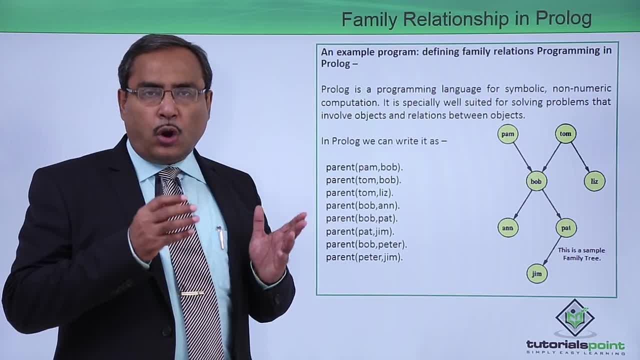 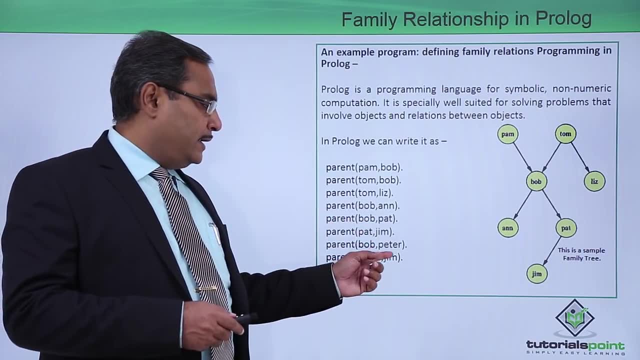 as the facts. that means the known knowledge base, So also known as knowledge base, also known as facts. So in this way, we have written this And this can also be under the category clause, and each and every clause must be terminated. 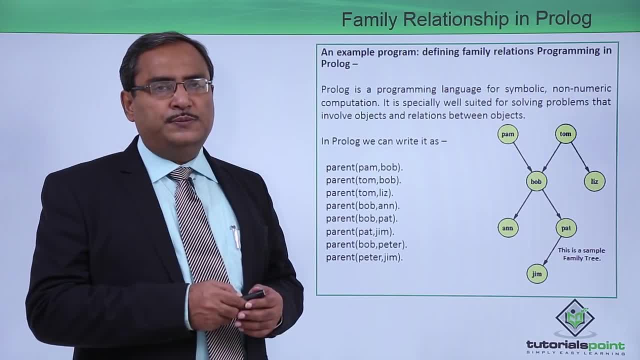 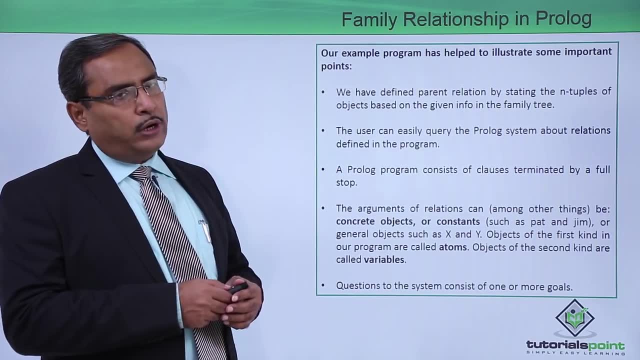 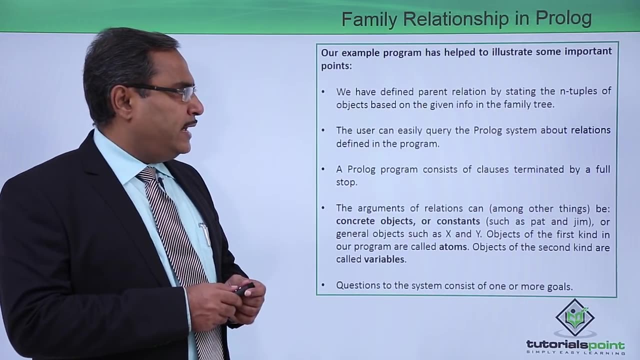 by a full stop, and that is the syntax of this Prolog language. So our example program has helped to demonstrate some important points. So what are the points we have noted here? We have defined parent relation by stating the n. tuples of objects based on the given. 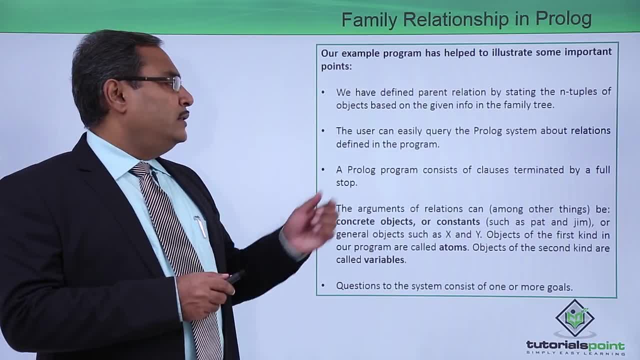 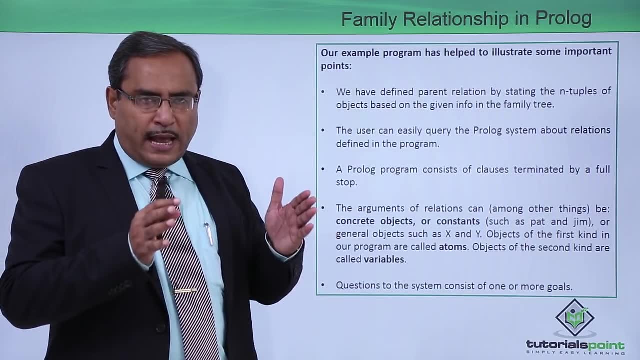 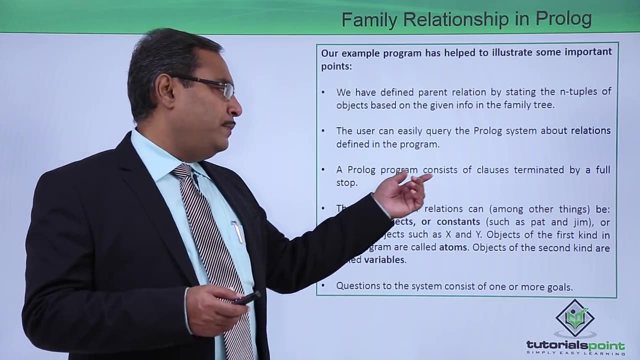 info in the family tree, The user can easily query the Prolog system about the relations defined in the program. So, whatever the knowledge base we are having, we can generate the respective queries and goals to get the answers. A Prolog program consists of clauses terminated by a full stop. as I mentioned earlier, The 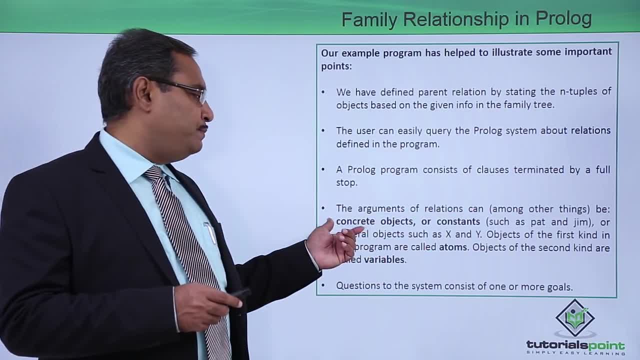 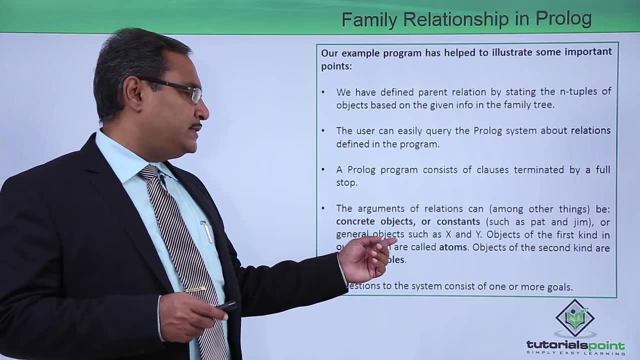 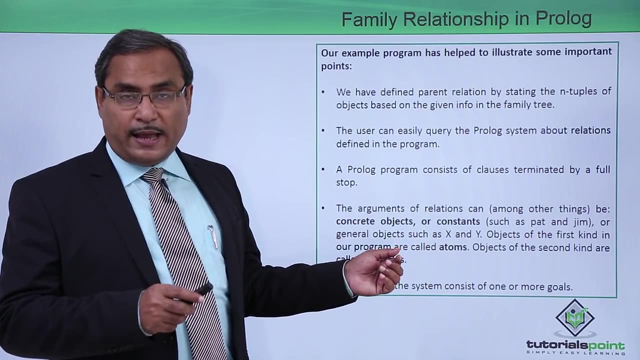 arguments of relations can among other things be concrete objects or constants, such as pat or gym, or general objects such as x and y. So here this x and x is written in capital and y is also written in capital, So they are the general objects can also be called: 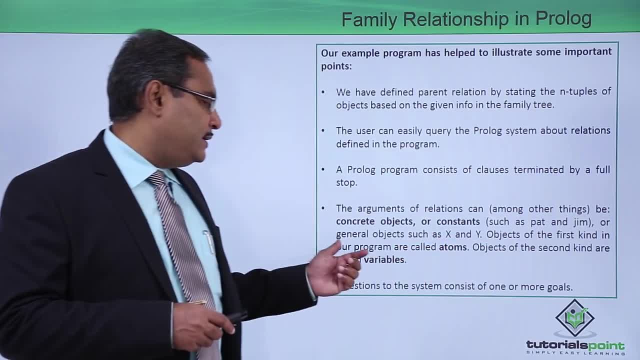 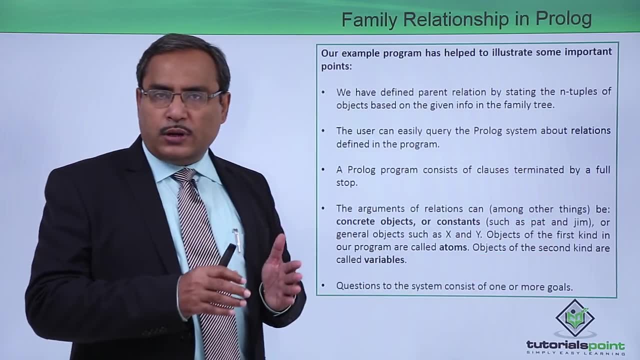 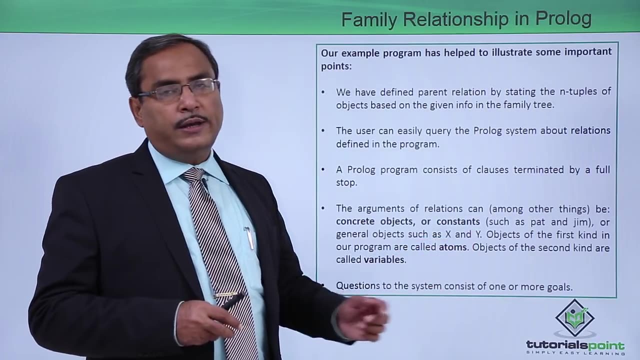 as variables. Objects of the first kind in our program are called atoms. So here we are having this: pat and gym. they will be known as the atoms, and objects of the second kind will be known as the variables. So here this, capital x and capital y will be known. 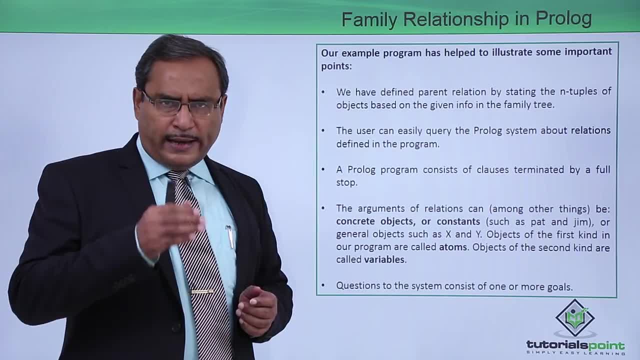 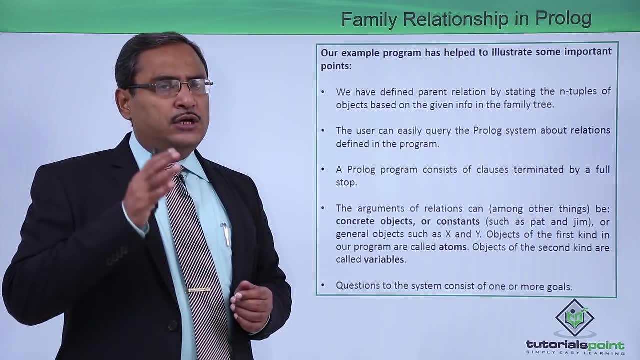 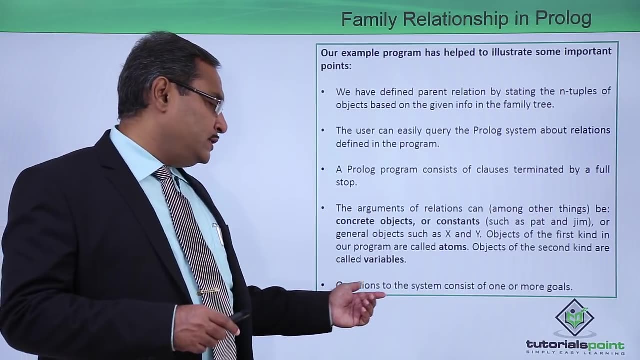 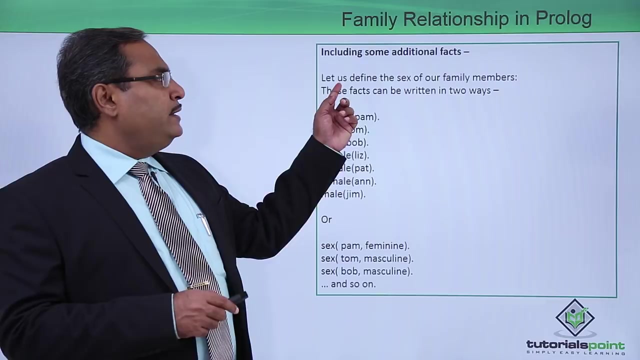 as the variables. So variables can be written in prologue, either starting with a capital letter or with one underscore. After that it may have smaller capital letter combinations, it can have underscore, it can have digits, and so on. Questions to the system consists of the one of the one or more goals, So let us define. 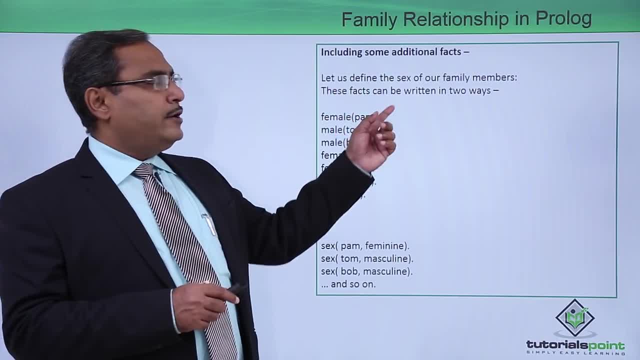 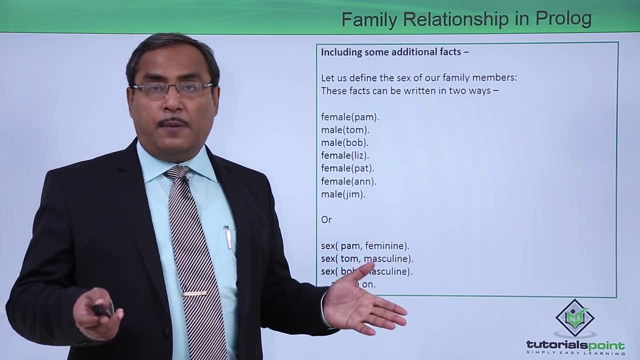 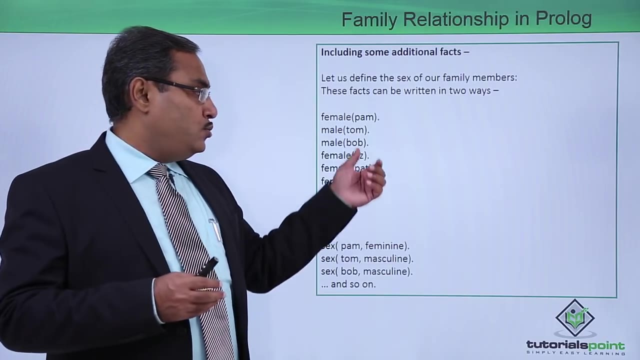 the sex of, the sex Sex of our family members. these facts can be written in two different ways. you can write in this way or you can write in this way, So that will depend upon your decision that how to define the sex of the family members using facts written in two different types. 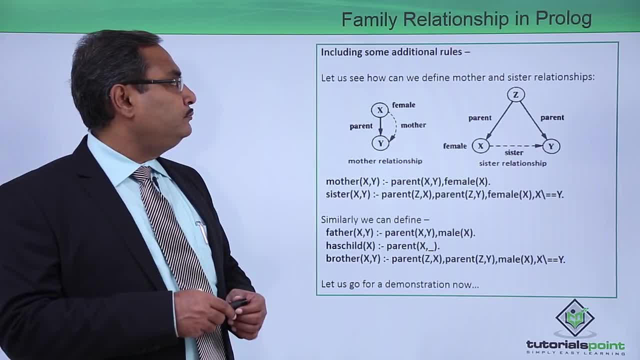 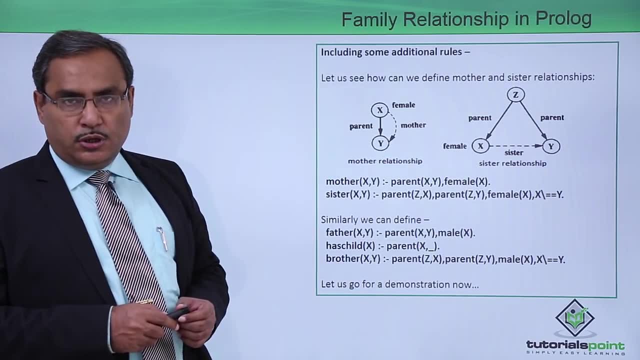 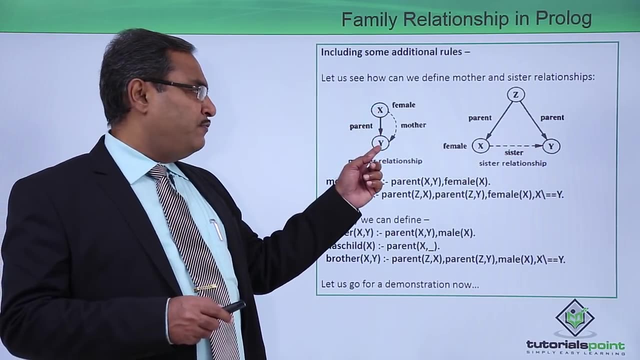 of clauses. you can select any one of them. So let us let us see how can we define mother and sister relationships. So how to define the mother relationship. x will be the mother of y if x is parent of y, along with x is female. 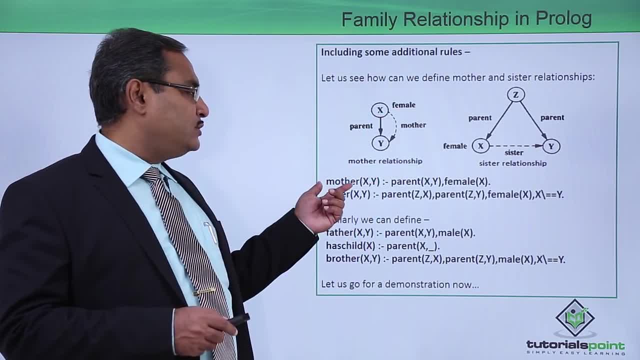 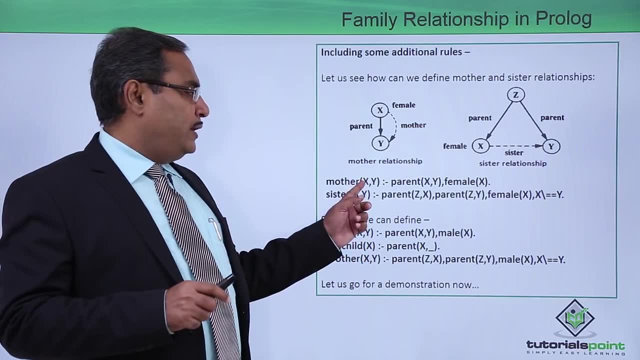 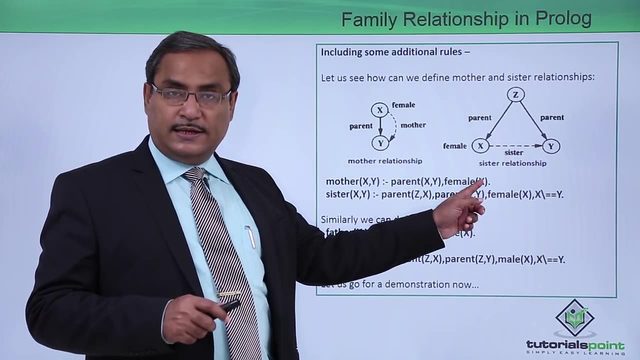 So how to write this one in prologue clauses? we can write in this way: x will be the mother of y here x and y are written in capital letters. that means they are the variables, So x and y. x will be the mother of y if parent x y and female x. So if two clauses are separated. 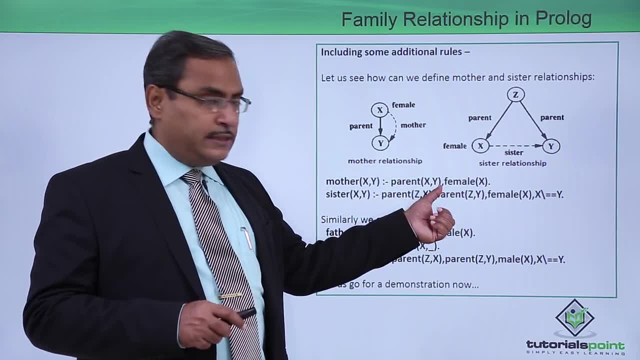 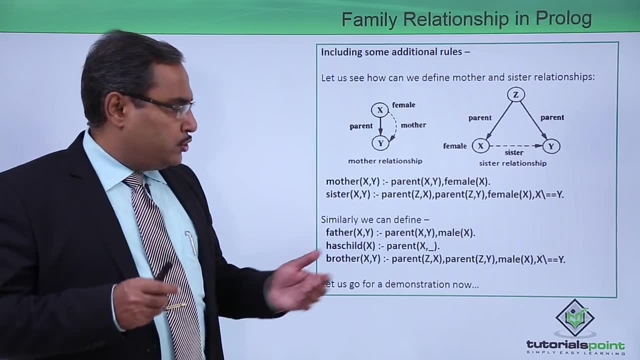 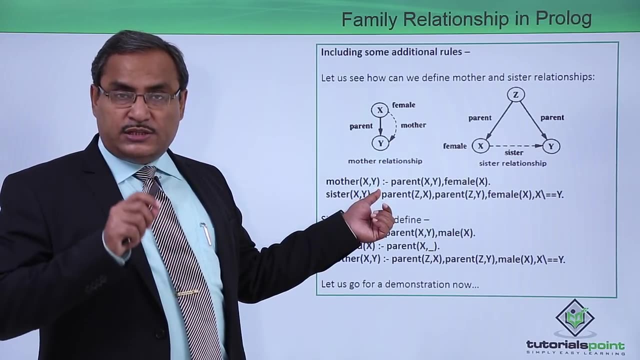 are satisfied at the same time, because here we are having this comma. comma denotes and, logic, So, on the other end, semicolon denotes or, So here these two conditions are connected by and, and this is known as if. colon dash is known as if, and each and every prologue. 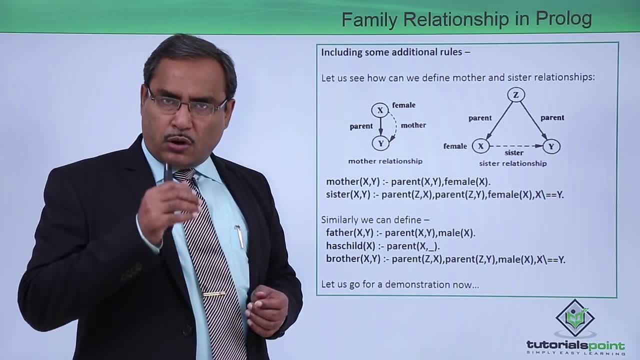 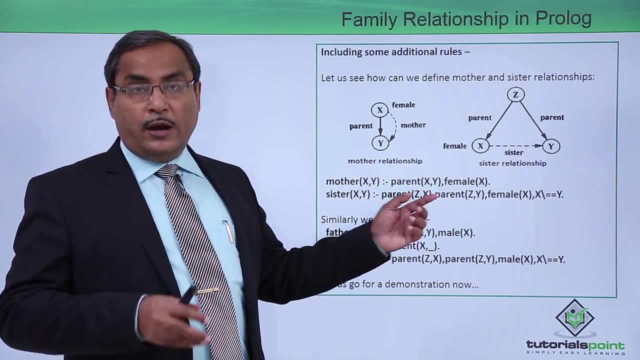 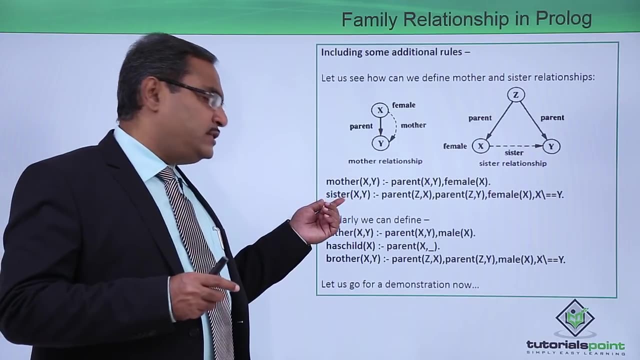 clause must be terminated by full stop. We know that clauses can be divided into two categories: one is the facts, another one is a rule. So this is our rule. and where we wrote something like your parent term pact. So that was our fact. that is a knowledge base. So, sister, how to define sister? So come to this diagram. 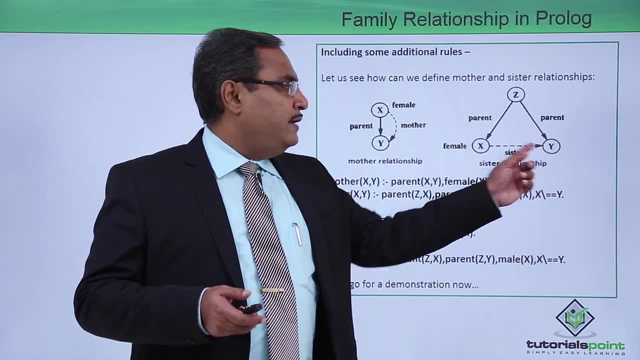 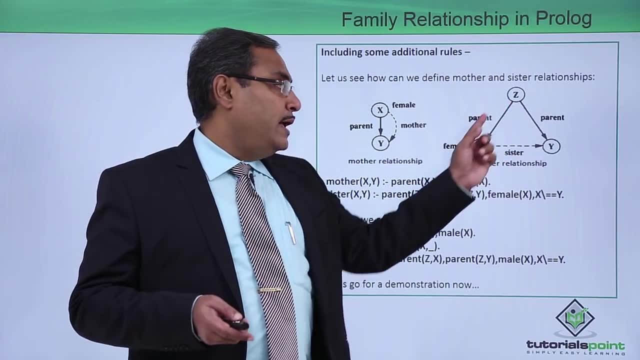 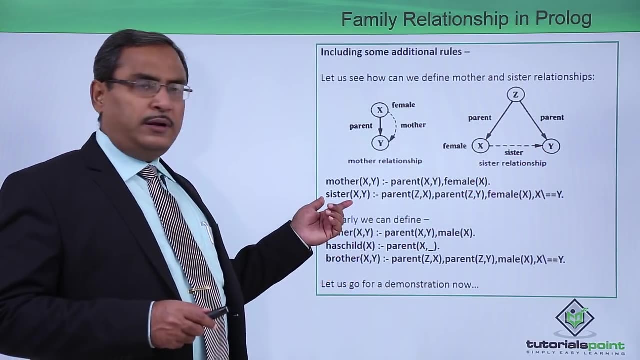 here. So x will be the sister of y if x and y, if they are having the same parent, let it be z also in the capital letters variable. and x is female for y. I need not to mention the respective sex for y. So how to write this one in prologue clauses? 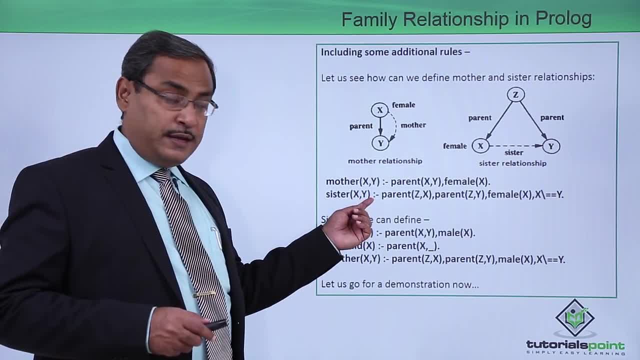 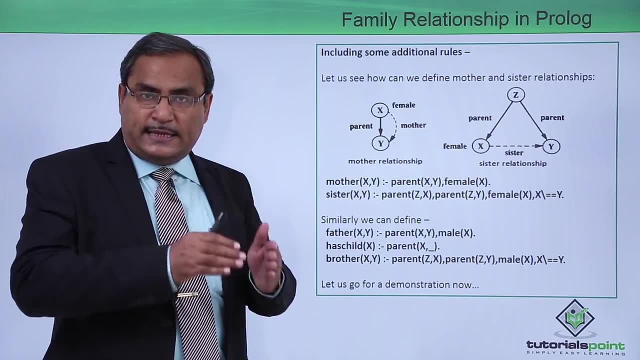 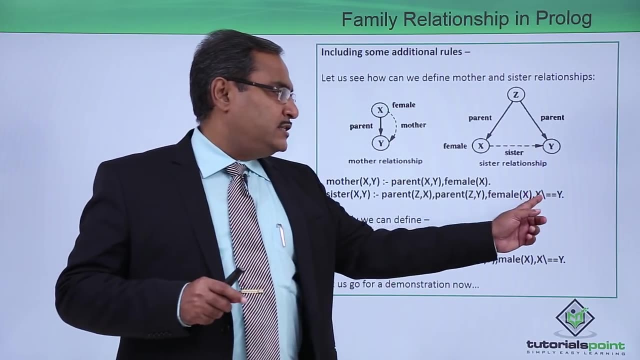 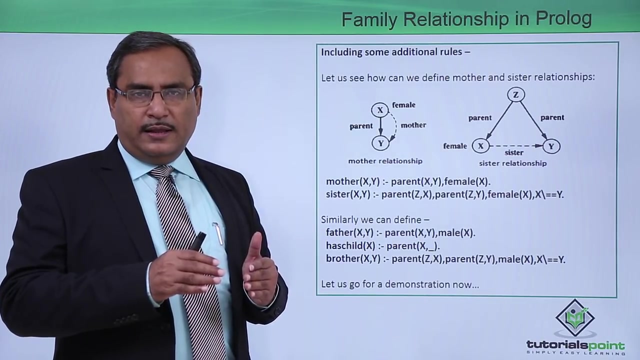 So sister x- y. if parent z x and parent z y, that means z is the common parent for x and y both, and female x last one, and x is not equal to y. So if x is not equal to y, x is a female and x and y both are having the same parent, let it be z, say. then you can. 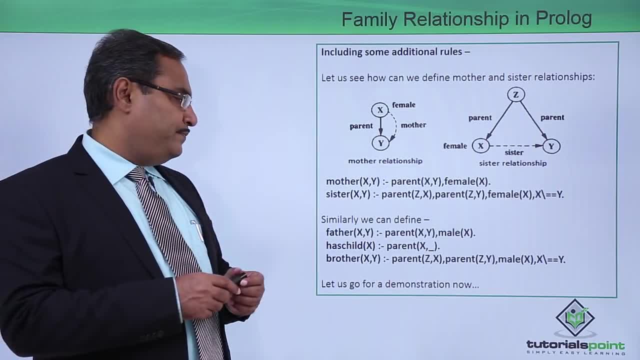 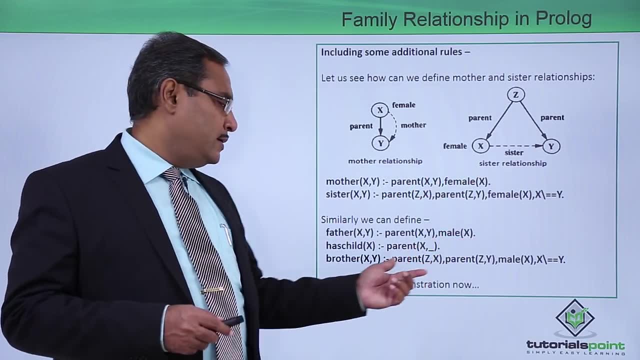 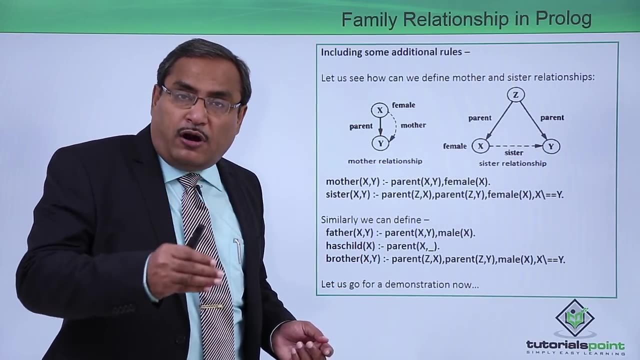 say that x is a sister of y. Similarly you can define the father. You can easily see that here we had the female, here we have written male And similarly we can also go for hash child. So x will have the child. if x is parent of someone, So someone. how to write someone? 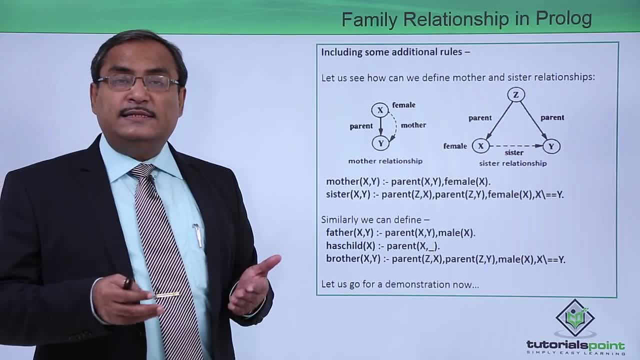 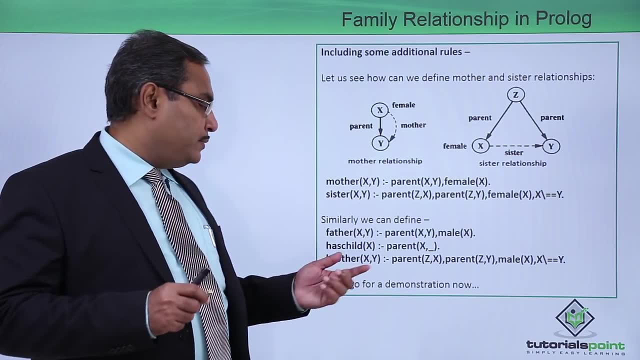 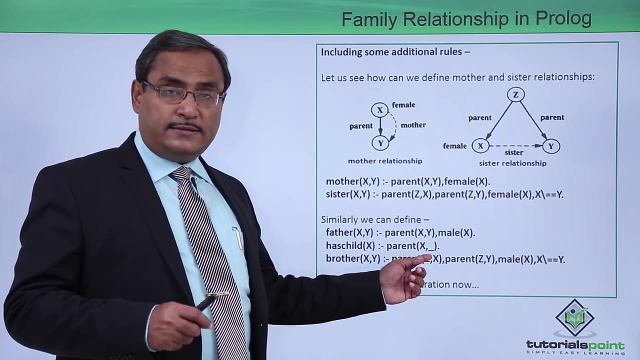 in prologue That is underscore. Underscore means what Means anonymous variable. So variable can be underscore and it is having a special meaning that it is anonymous variable. So brother x- y. So we have defined sister Now brother x- y. So parent x z, parent z x, rather. 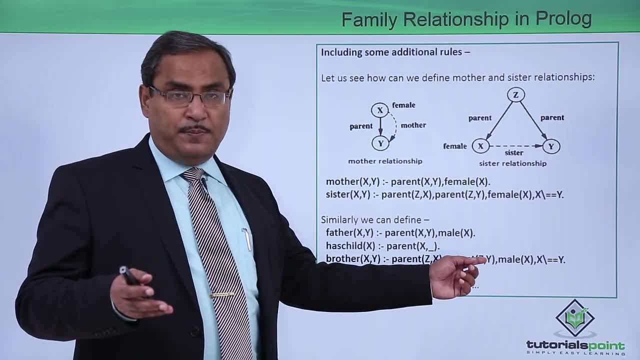 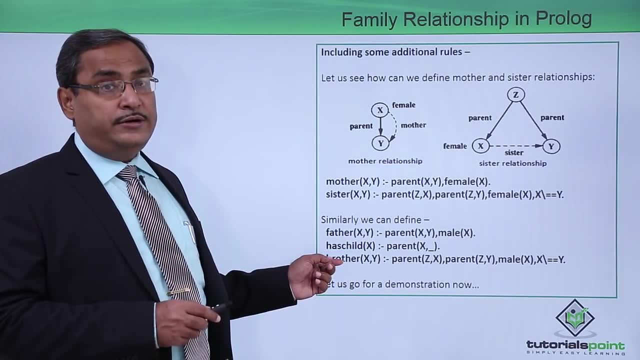 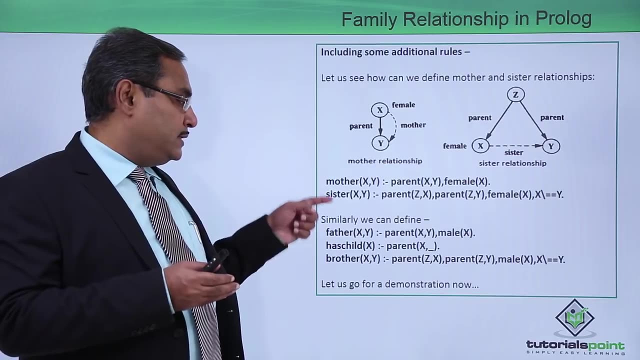 and parent z, y. So that means the same parent for x and y, And male x and x is not equal to y. So in this way also you can define brother relation. So where we have defined our parent, our sex relation, then mother, sister. 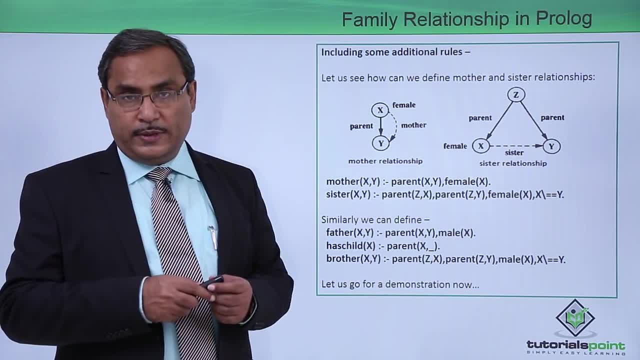 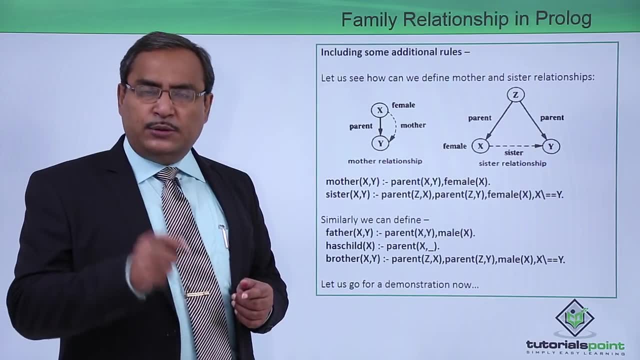 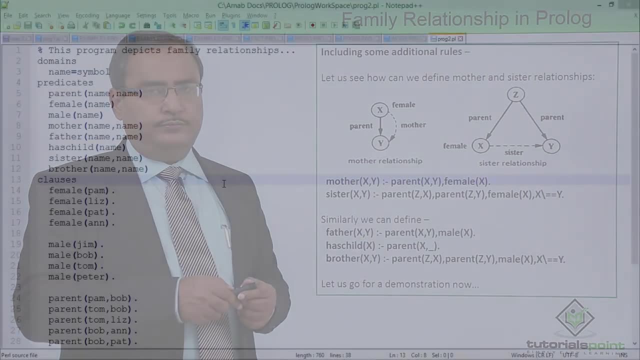 Father, hash child, brother and so on. So let us go for the practical demonstration, for the better understanding how this code should be written and how to execute them through certain queries or goals. So here is the demonstration for you. This is a sample prologue program. 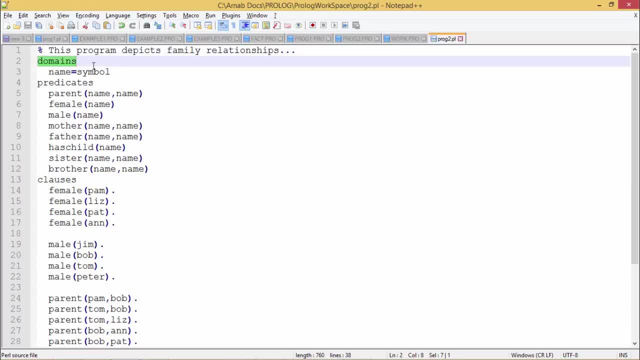 A prologue. program will have mainly three sections: One is the domains, next one is the predicates and the last one is the clauses. So under domains we will be having name is equal to symbol or some sort of declarations like this: 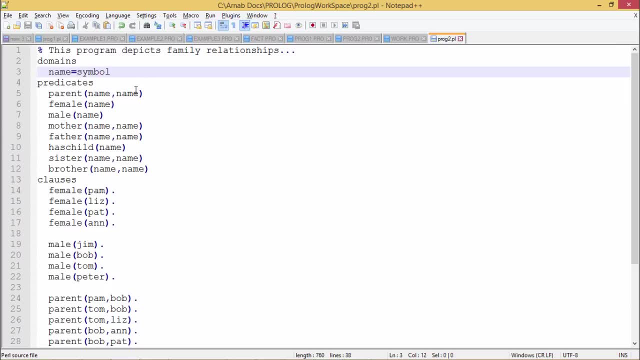 Where symbol indicates that it is of the type text or string And name. this is my keyword, my word. I have given We can use some other names here also. No issues. So predicates under the predicates: we shall be declaring all the predicates under which the clauses will be. 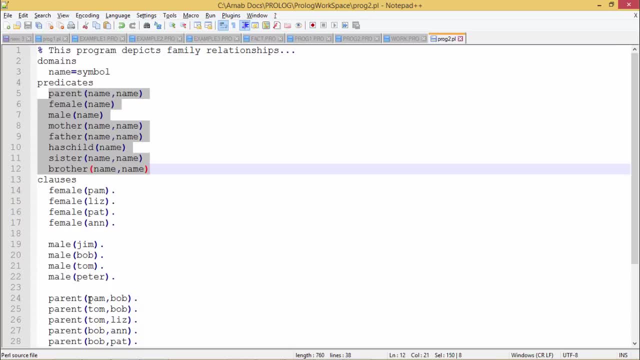 defined. So here we are having this parent, So fam and parent, So we are having this parent. So we have written this one like this: parent name, common name, female name and so on, Under the clauses' sections we shall discuss or we shall define our databases. So this is our farewell friend. 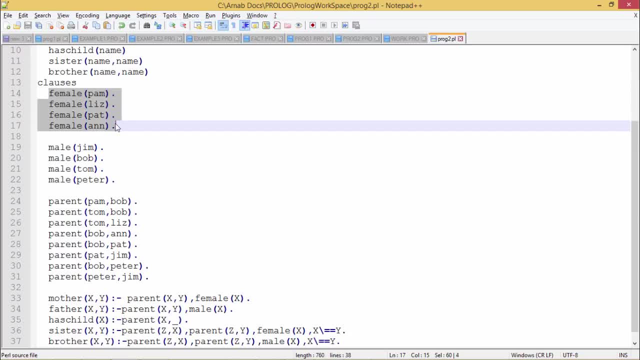 who is female and please that. and all of them are female. So here I'm declaring some other knowledge base- and this is the respective knowledge- is quite different. Is it the cloth? And this is that the first class __________. 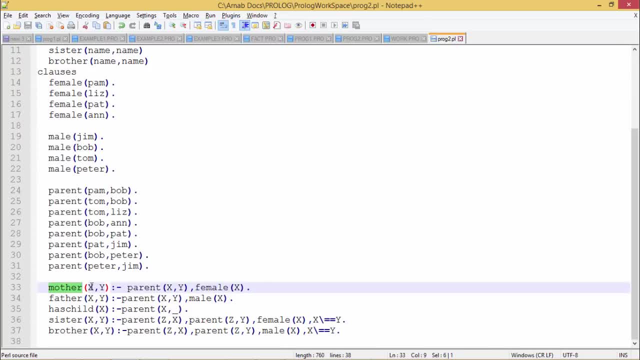 __________ here is known as the mother. so mother X, comma Y. so you see, under clauses we are writing such. these are known as the rules, these are known as the rules and this clauses will be known as the facts. okay, so facts and rules will be the 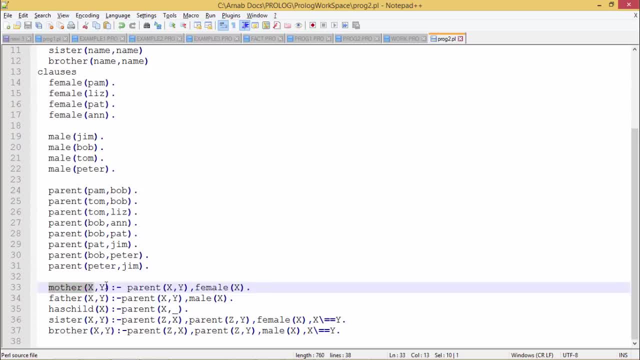 members of the respective clauses. so mother X comma Y. this symbol indicates if, and this comma indicates and, and full stop or period will be indicating the terminating of the respective clauses. okay now. so mother X comma Y. if parent X comma Y comma means and female X. in this way we have defined, father has child. 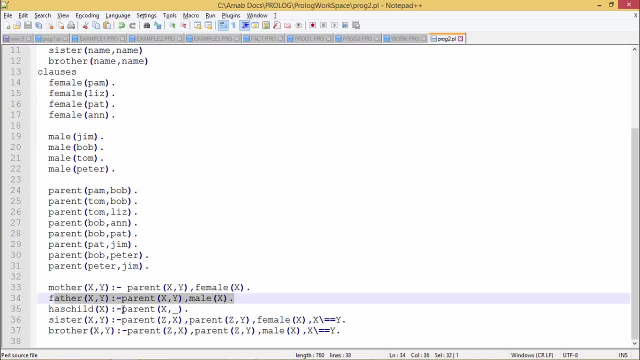 means X will have a child. if if parent X comma underscore here under code underscore indicates that mother X comma Y will have a child. if parent X comma means that it is anonymous variable sister X comma Y. if parent Z comma X, parent Z comma Y, that means if Z is the common parent for X and Y and if female. 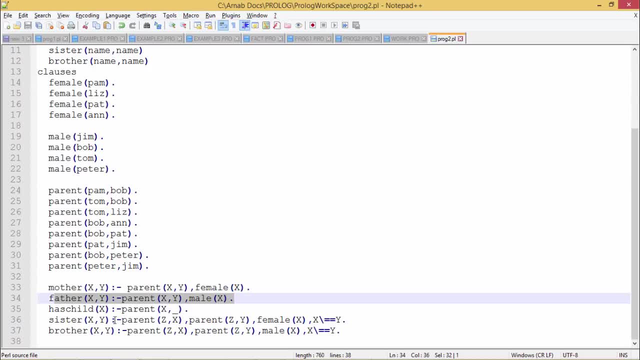 X then and X is not equal to Y, then we shall say that sister XY is working in other versions of prologue instead of having this operator. we can also use the operator like this one in other versions of prologue, but in case of G, a new prologue will be going for this operator. so, similarly, we 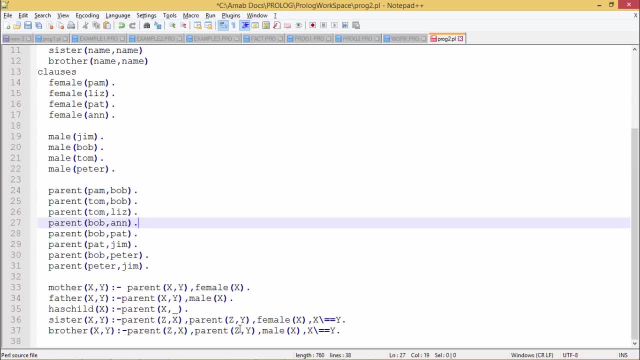 have defined this: brother, parent Z X, parent Z Y and male. X and male and X is not equal to Y. so in this way we have defined the respective facts. these are the facts and these are the rules under the section clauses. but in case of G a, 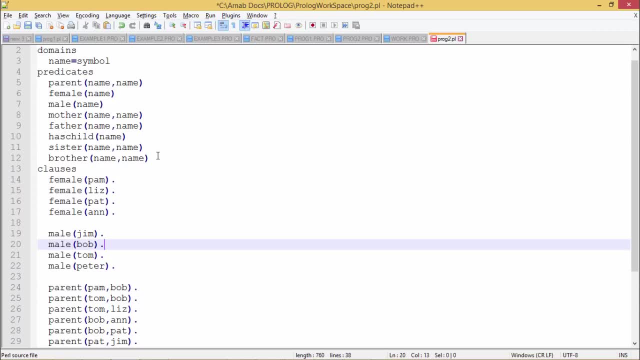 new prologue, these clauses, predicates and domains. these sections are not required, so that's why we are putting them under block comment. so in case of prologue, we can write comments in two different ways. in case of single line comment, it can be preceded by the percentage symbol. in case of block: 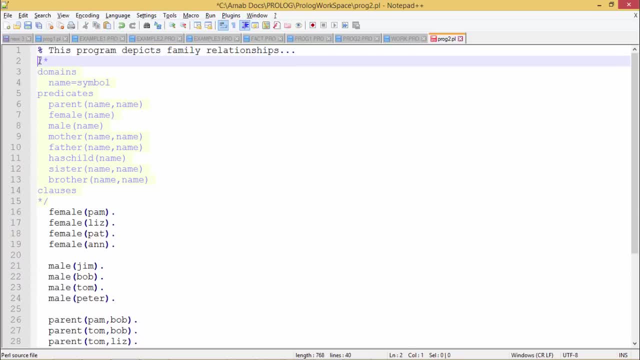 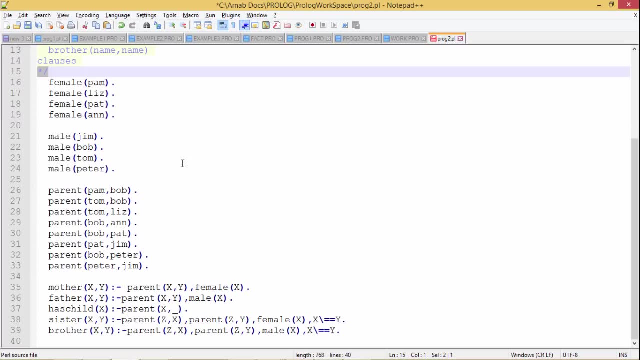 comment. it should be. it should be enclosing the total block under slash star and star slash in this way. okay, so we are having this female male parent, mother, father has child, sister and brother in this way, so now let us go for the respective execution. here we have. 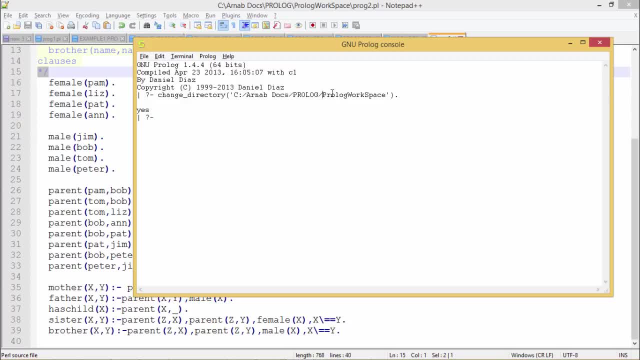 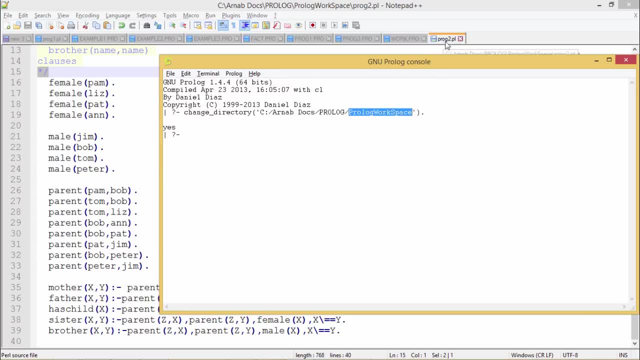 already done the change directory. so under this particular folder, that is prologue workspace- under this particular folder, prologue workspace, we have saved this file that is proc2.pl. so now the program has been compiled, and it has been. it has found that no error is there, so it is executable now. 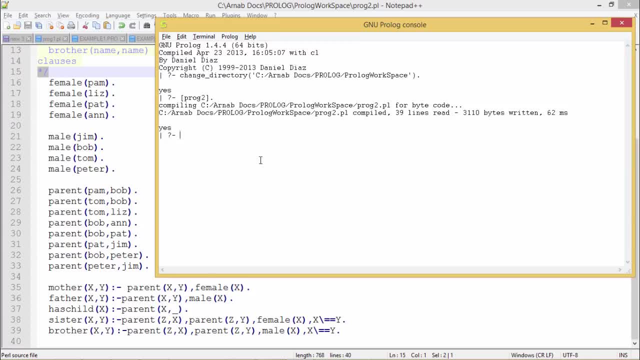 so now let me execute with some respective goals. so I'm going for. we know that in case of variables, the variable name must be starting with some capital letters. so now, if I want to have any other options pending, then I can give semicolon there and here we are getting two. one is Pat, another one 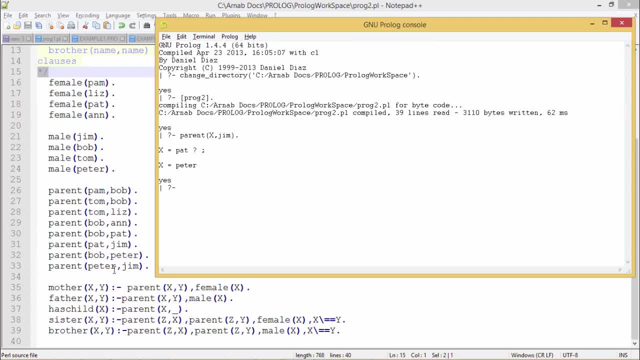 is a Peter. let me check. so Jim, so Pat, Jim, Jim, so it is Peter, Jim. so that's why you got two answers. now let me go for mother. if I want to terminate the solution here, then I can press enter, I can hit enter. but if I want to get all other combinations, then I can, I can press.